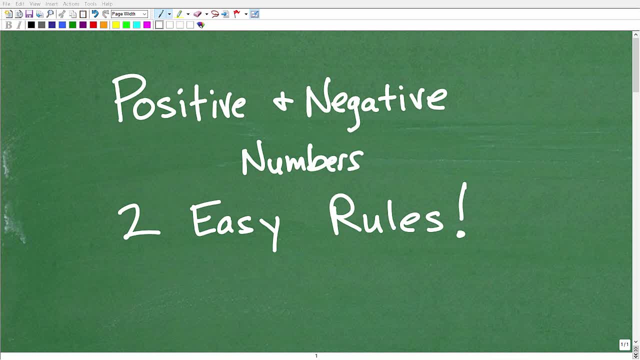 Okay, let's talk about positive and negative numbers. This is probably one of the top- I would say top five- areas where students get math problems. wrong is they simply don't know their positive and negative number rules as well as they think. Okay, so the whole purpose of this video is to, you know, dispel any confusion. 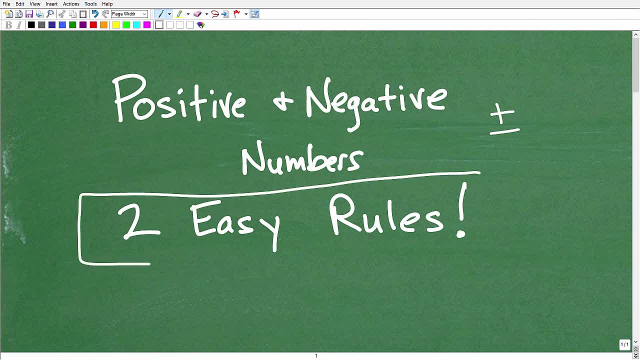 and give you two easy rules that you will never make a mistake again, with positive and negative numbers. So that is the goal. Now, before we get started here, let me go ahead and introduce myself. My name is John. I'm the founder of Tablet Class Math. 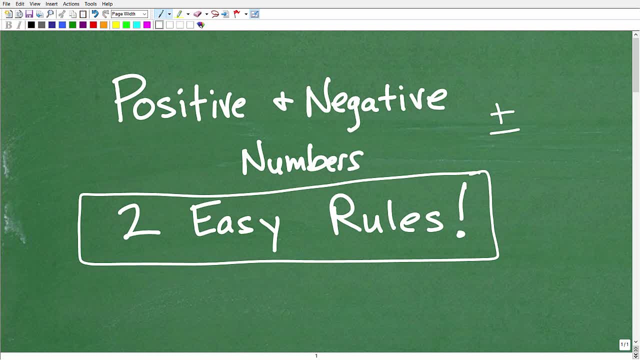 I'm also a middle and high school math teacher And if you really want to learn math from me, I'm going to encourage you to check out my math learning program. I'm going to leave a link to that in the description of this video. 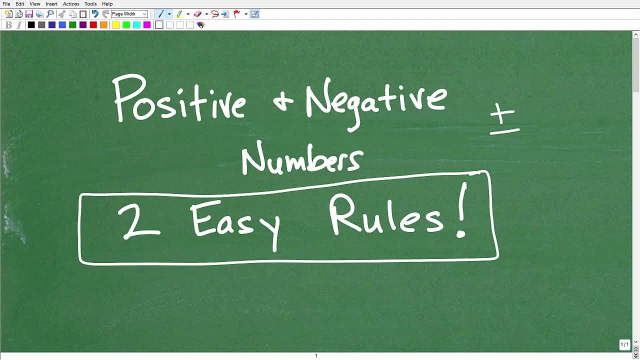 I have over over a hundred plus courses, So whatever math that you're taking likely can help you out. So I'm going to again leave a link to my math program in the description of the video. And also I've been on YouTube for several years. 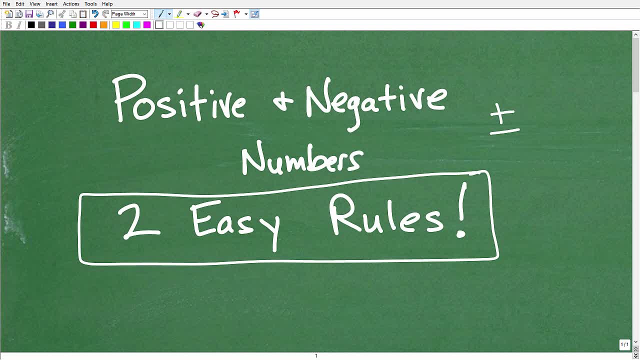 I have hundreds and hundreds of math videos that can help you out in various levels of mathematics, So hopefully you'll consider subscribing And, of course, if this video helps you out, please give it a thumbs up and give me some feedback in the comments section. 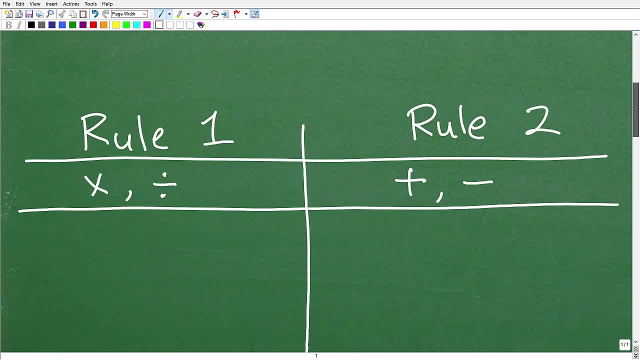 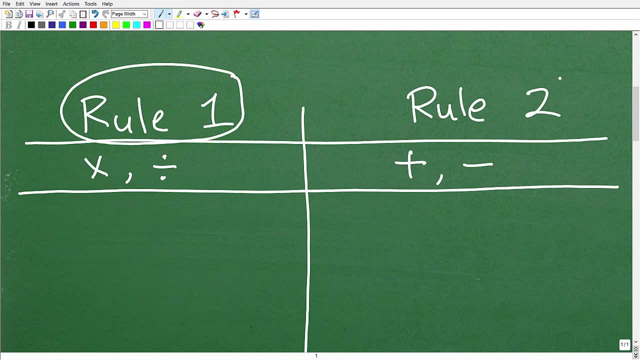 All right, Let's get to it. All right, So two easy rules, All right. So here we have one rule, We'll call this rule one, And then we've got this other rule over here, rule two. Let's go ahead and start with rule one. 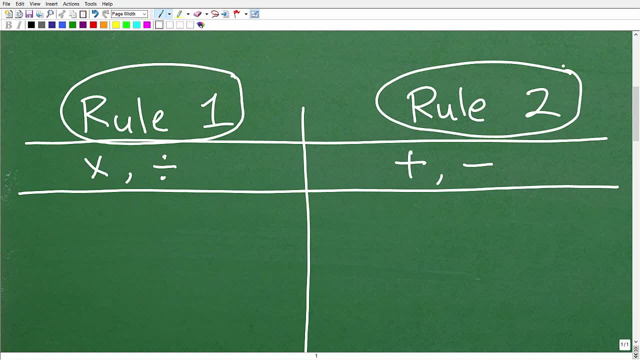 Okay, So rule one will cover positive and negative numbers when we have multiplication or division going on. Okay, So let's look at an example. This is very, very simple. So if I have negative two times Negative two, the answer is what? 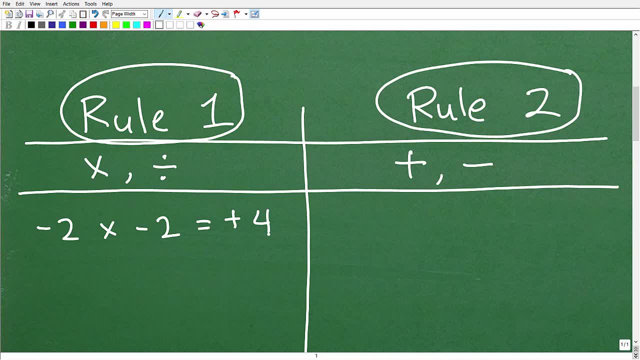 Well, hopefully you already know that it's going to be a positive four. Okay, So if the rule goes like this: if the signs are the same, Okay, So we have a negative here and a negative here, So same. Let's do it this way. 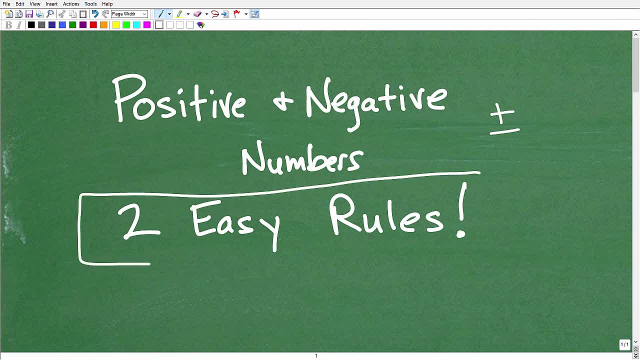 and give you two easy rules that you will never make a mistake again, with positive and negative numbers. So that is the goal. Now, before we get started here, let me go ahead and introduce myself. My name is John. I'm the founder of Tablet Class Math. 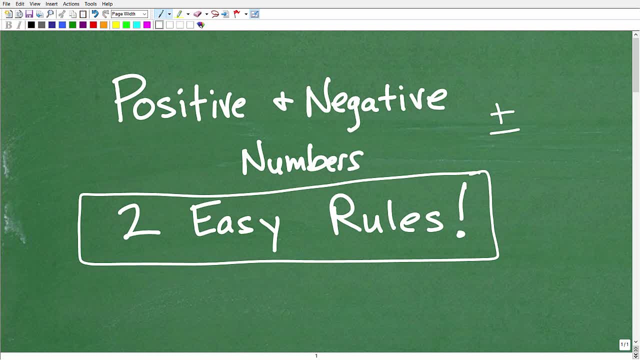 I'm also a middle and high school math teacher And if you really want to learn math from me, I'm going to encourage you to check out my math learning program. I'm going to leave a link to that in the description of this video. 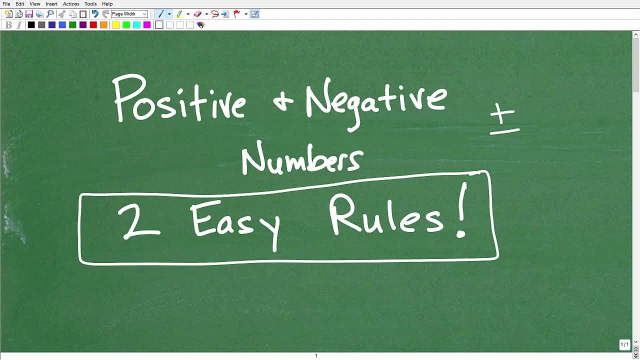 I have over over a hundred plus courses, So whatever math that you're taking likely can help you out. So I'm going to again leave a link to my math program in the description of the video. And also I've been on YouTube for several years. 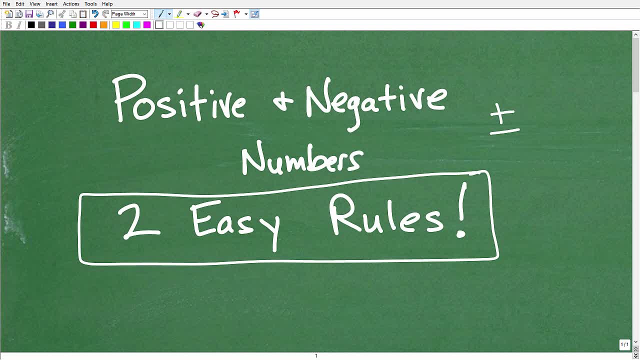 I have hundreds and hundreds of math videos that can help you out in various levels of mathematics, So hopefully you'll consider subscribing And, of course, if this video helps you out, please give it a thumbs up and give me some feedback in the comments section. 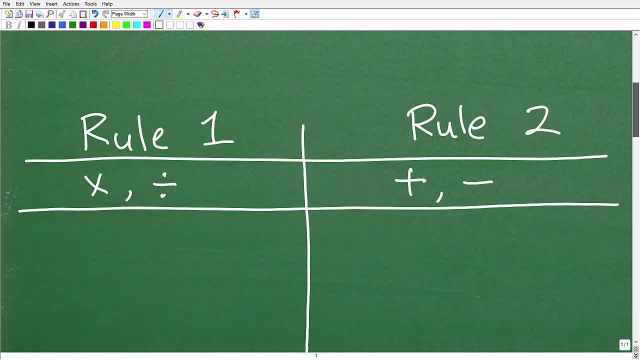 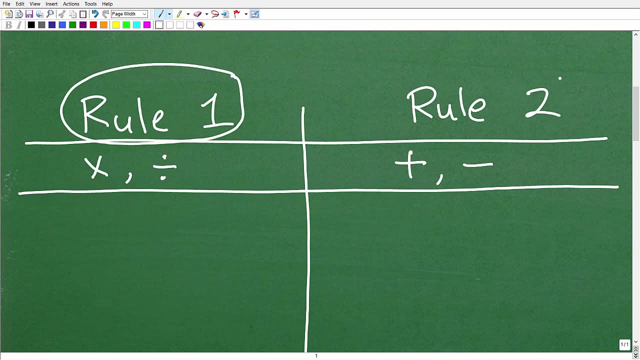 All right, Let's get to it. All right, So two easy rules, All right. So here we have one rule, We'll call this rule one, And then we've got this other rule over here, rule two. Let's go ahead and start with rule one. 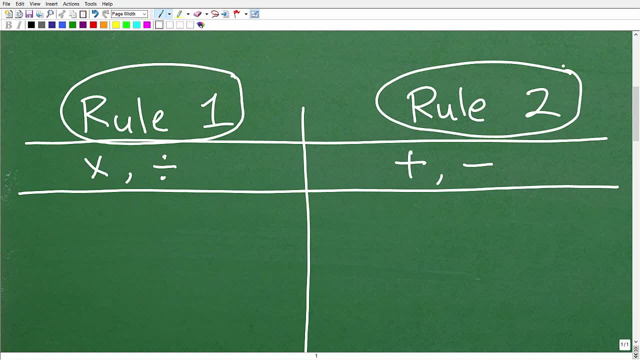 Okay, So rule one will cover positive and negative numbers when we have multiplication or division going on. Okay, So let's look at an example. This is very, very simple. So if I have negative two times Negative, two times negative two, the answer is what? 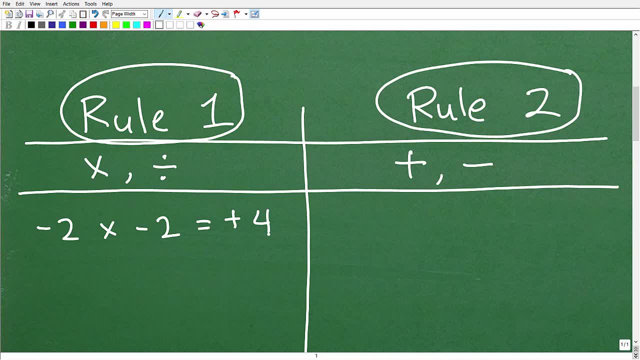 Well, hopefully you already know that it's going to be a positive four. Okay, So if the rule goes like this: if the signs are the same, Okay, So we have a negative here and a negative here, So same. Let's do it this way. 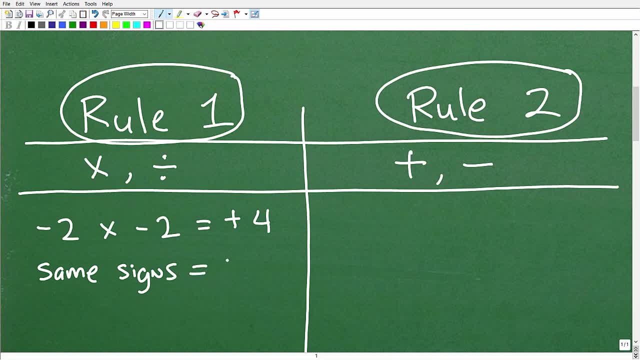 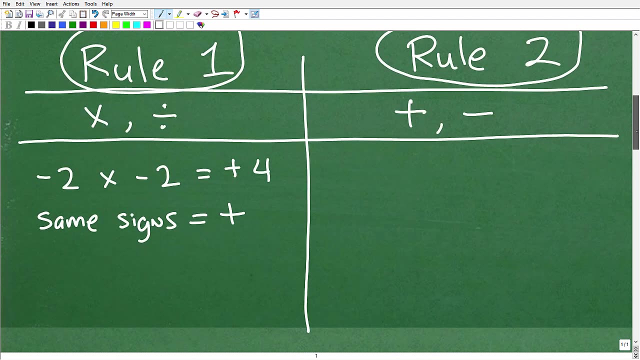 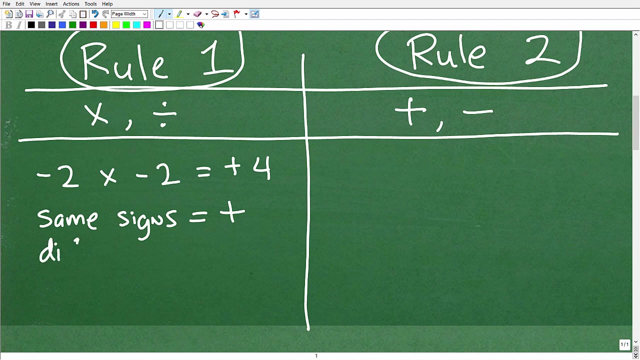 Same signs, Our answer is going to be positive all the time. So this is a positive two times A positive two. we have a positive four. Negative two times a negative two going to be a positive four. Okay, And the rule: okay, obviously, if the signs are different. so let's go like this: different signs. 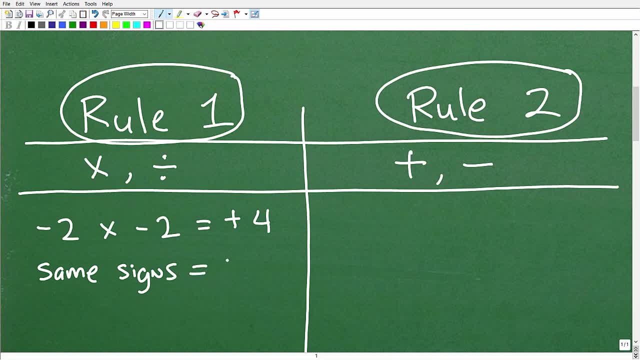 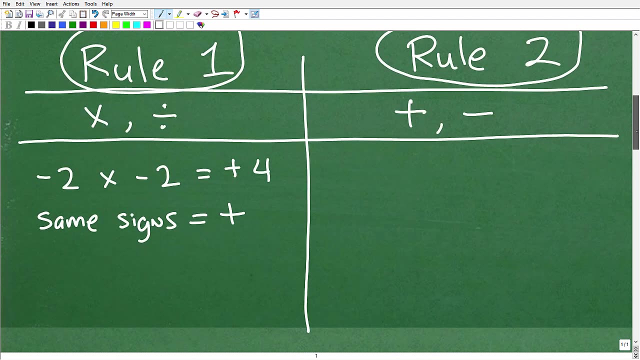 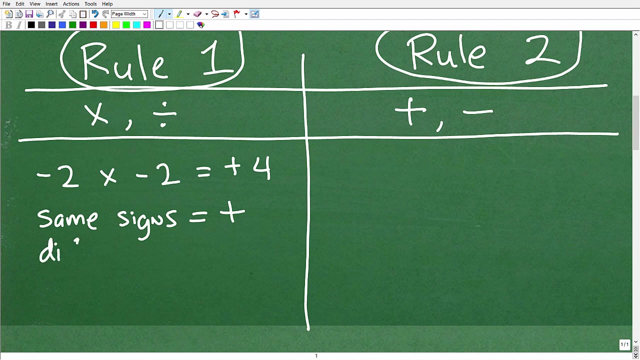 Same signs, Our answer is going to be positive all the time. So this is a positive two times A positive two. we have positive four. Negative two times a negative two. going to be a positive four. Okay, And the rule: okay, obviously, if the signs are different. so let's go like this: different signs. 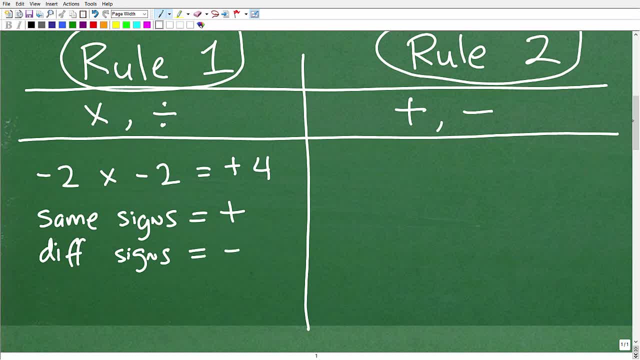 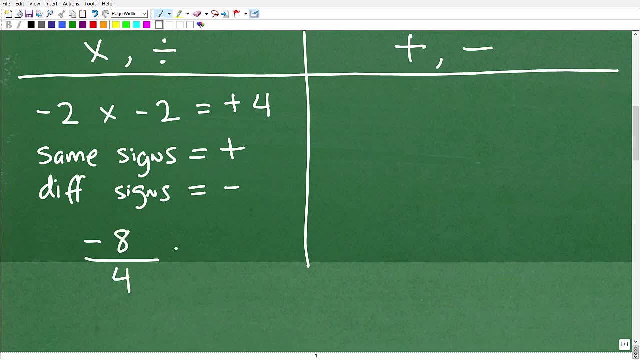 All right, Then the answer will be a negative. So let's take a look at something like this: Negative eight divided by a positive four. Okay, So here, this is negative, This is positive. All right, So when we do this division, our answer is obviously going to be two. 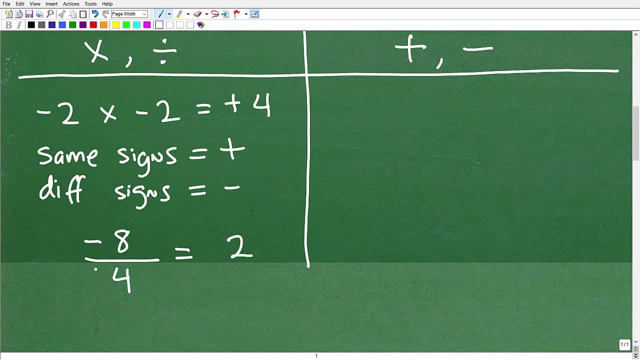 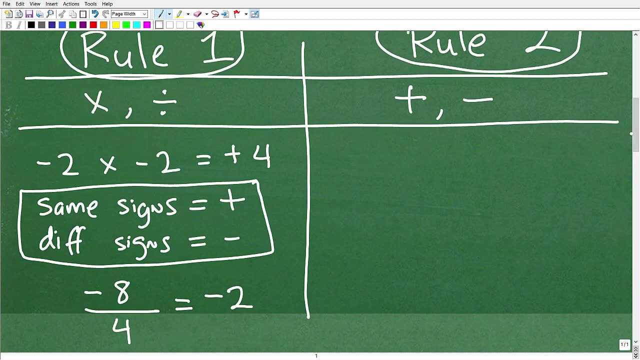 But what is the sign? The signs are different, The numbers here are different, So my answer is going to be negative. So this rule right here applies to both multiplication and division. Super easy And if you can remember this, okay, this covers what? 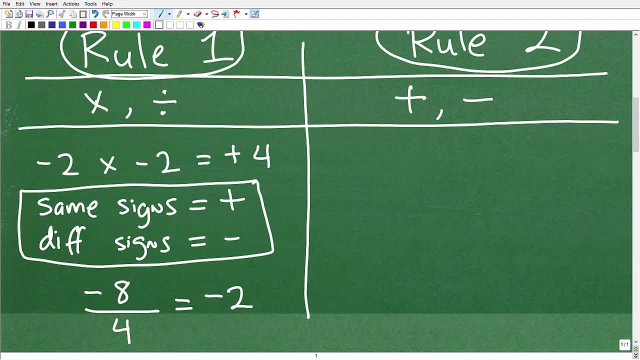 Fifty percent of the math operations that you're doing. So we just We just covered multiplication and division situations. okay, Very, very easy, All right. So hopefully, you know, take notes, you know remember this because, again, it's an easy rule. 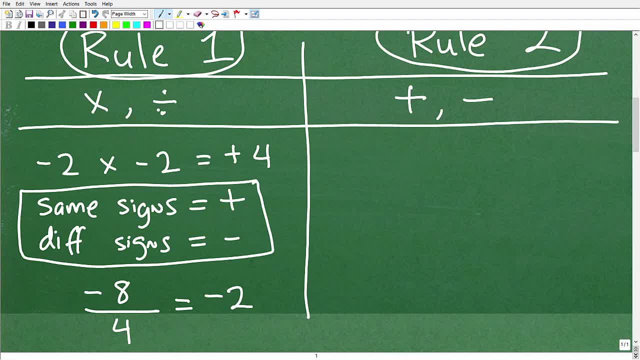 but it's also easy to forget. okay, Do not rely just solely on your calculator or your mental memory. When you're kind of mastering this, like double check yourself, right When you're doing your homework or whatnot, you know you'd be like, okay, wait a minute. 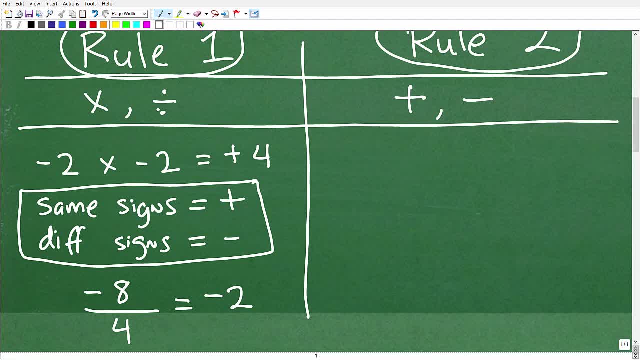 Am I doing this correct? You know, have this little on like you know rule rules here, like on a three by five index card or in your notes. That way you can always make sure that you're kind of creating the right math habits in your brain. 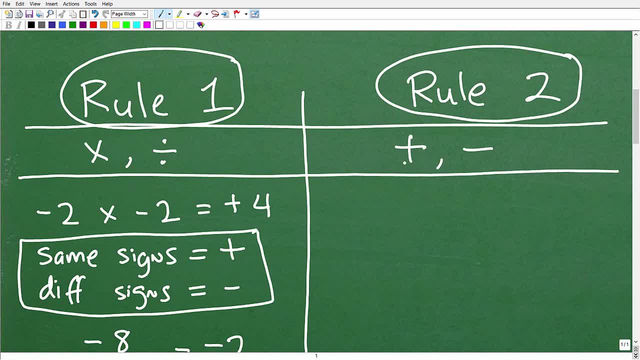 All right, So let's go on to rule number two, And this is going to cover addition and subtraction situations. So, basically, this rule is the same. So if you know how to add or subtract, you're basically We're doing the same thing here, okay. 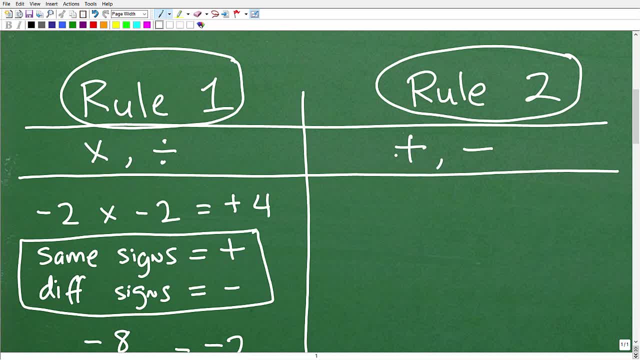 Okay, Now this one is going to be a little bit more involved, And I think this is where students kind of find positive, negative number concepts a little bit more confusing. But here's, I'm going to give you a way to think about this rule. okay, that's nice and easy. 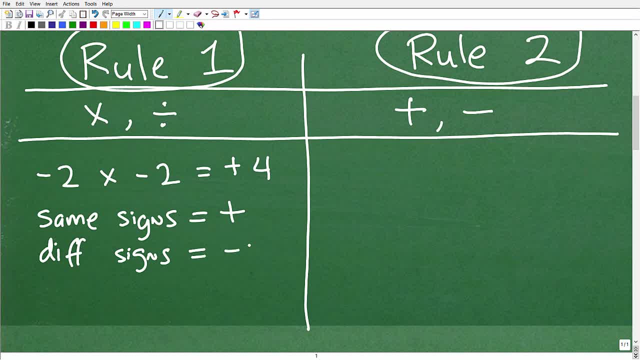 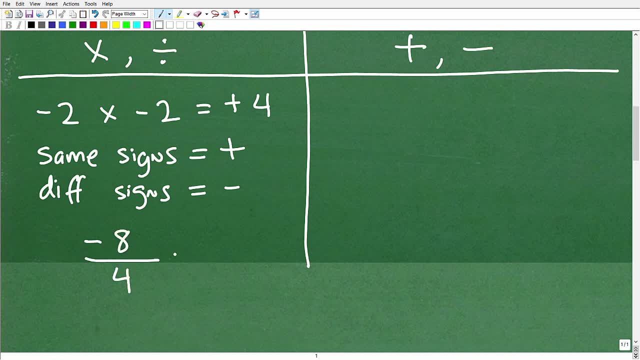 All right, Then the answer will be a negative. So let's take a look at something like this: Negative eight divided by a positive four. Okay, So here, this is negative, This is positive. All right, So when we do this division, our answer is obviously going to be two. 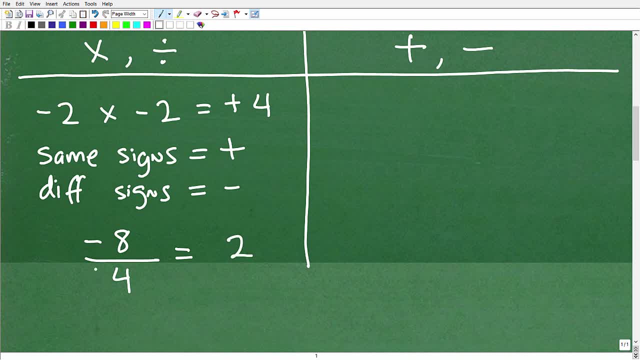 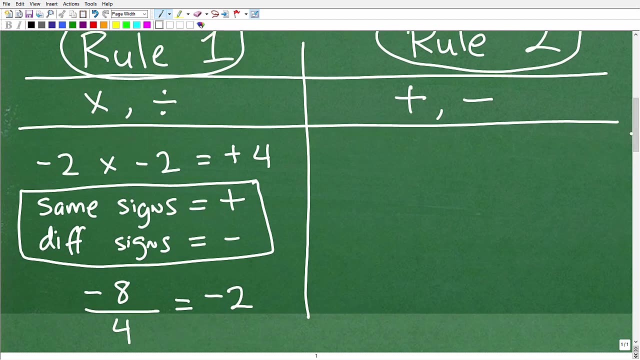 But what is the sign? The signs are different, The numbers here are different, So my answer is going to be negative. So this rule right here applies to both multiplication and division. Super easy And if you can remember this, okay, this covers what 50% of the math operations that you're doing. 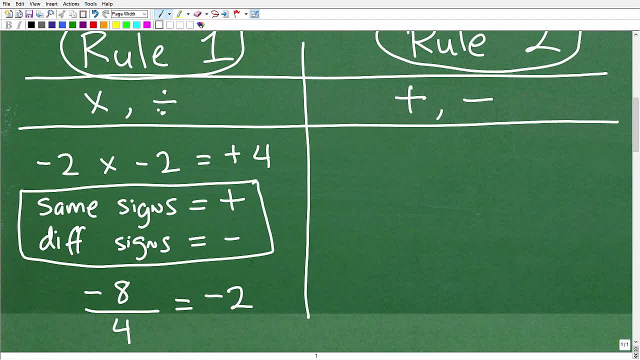 So we just, We just covered multiplication and division situations. okay, Very, very easy, All right. So hopefully, you know, take notes, you know, remember this because, again, it's an easy rule but it's also easy to forget. 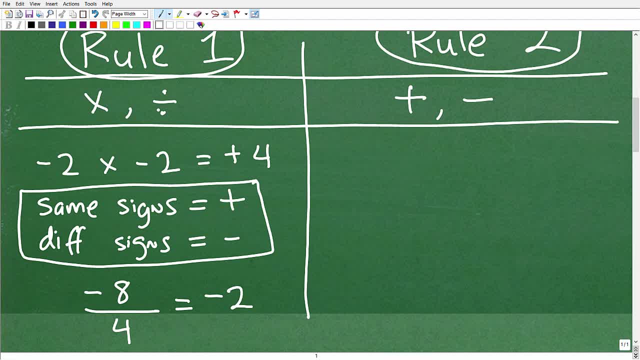 Okay, Do not rely just solely on your calculator or your mental memory. When you're kind of mastering this, like double check yourself, right When you're doing your homework or whatnot, You know you'd be like: okay, wait a minute. 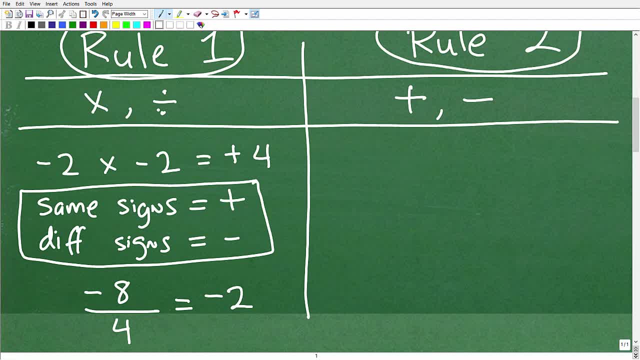 Am I doing this correct? You know, have this little on like you know rule rules here, like on a three by five index card or in your notes. That way you can always make sure that you're kind of creating the right math habits in your brain. 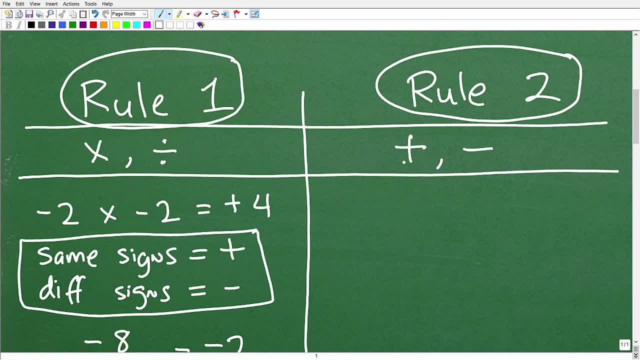 All right. So let's go on to rule number two, and this is going to cover addition and subtraction situations. So, basically, this rule is the same. So if you know how to add or subtract, you're basically we're doing the same thing here. 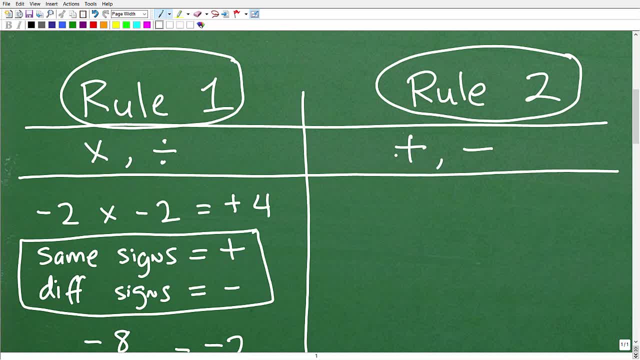 Okay, Now this one is going to be a little bit more involved, and I think this is where students kind of um, find positive, negative, number, uh- concepts a little bit more confusing. but here's, I'm going to give you a way to to think about this rule. 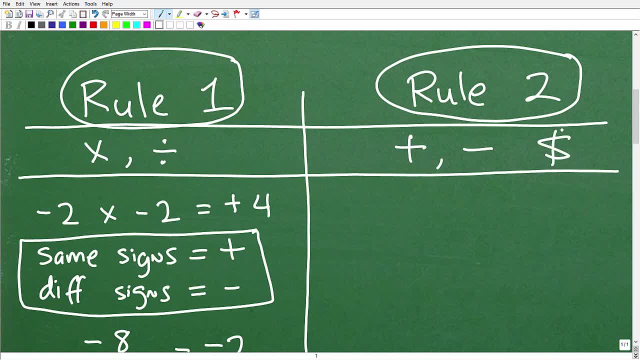 Okay, That's nice and easy, And we're going to use the concept of money, right? Everyone's favorite topic, So let's let's talk about money. All right, Let's use money as our model here. for rule two. 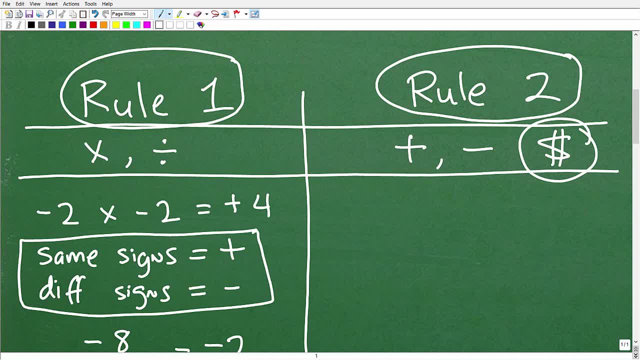 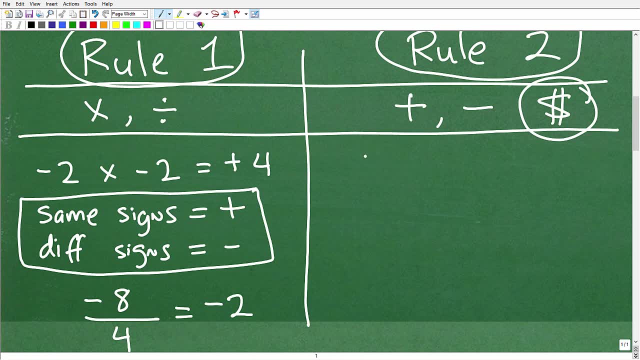 Okay, So, uh, the second rule, okay, Rule number two here. All right. So how is this going to work? Just let's, let's think of money, um, in this manner, All right, So let's say we have a positive three. 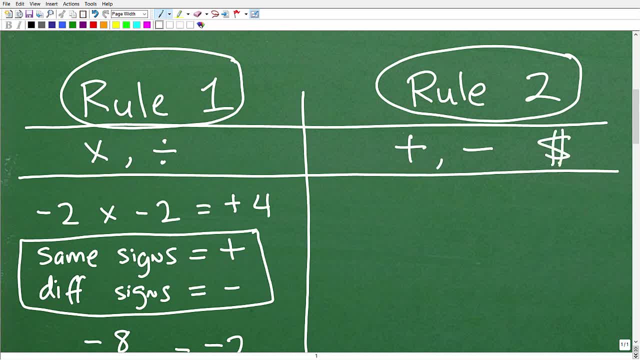 And we're going to use the concept of money, right, Everyone's favorite topic, So let's talk about money. all right, Let's use money as our model here. for rules, Let's use the second rule. okay, Rule number two here. 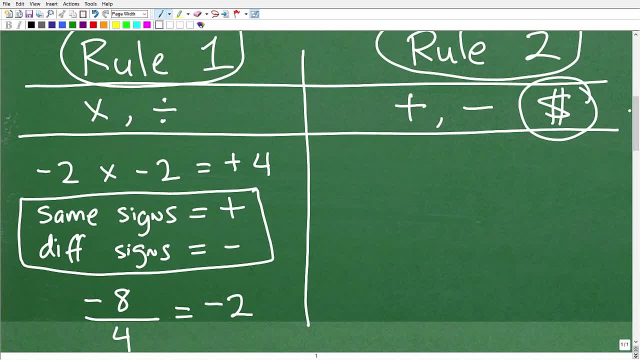 All right. So how is this going to work? Just let's think of money in this manner. all right, So let's say we have a positive three, okay, And we're going to add it to seven, all right. So when we have a positive number, we don't need to write a little positive sign like this. 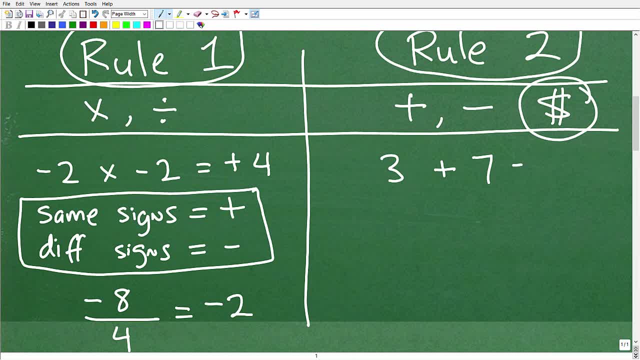 So this is positive three plus a positive seven. So this is just simple addition, right? So the answer is Now. I want you to think of this in terms of a dollar situation. okay, So this is like having three dollars, okay. 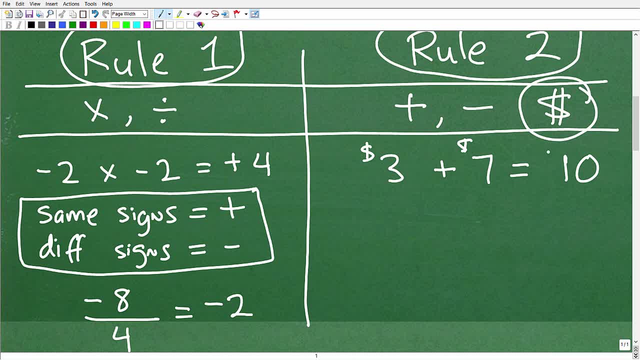 At the end, someone gives you seven dollars, So in total you have ten dollars. So that's pretty cool, right? All right, Now let's kind of change this around. all right, Let's put: Instead of having positive signs here, let's think of this in terms of negative signs. 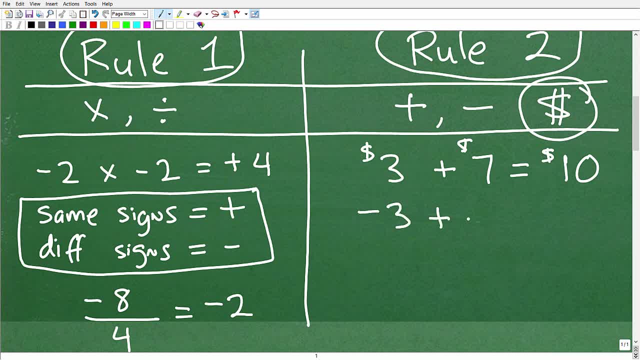 So let's have negative three, So negative three plus negative seven, and now let's figure out what this answer is going to be. okay, Now, negative three. all right If I have negative three dollars. okay Again, we're trying to use money here as our model. 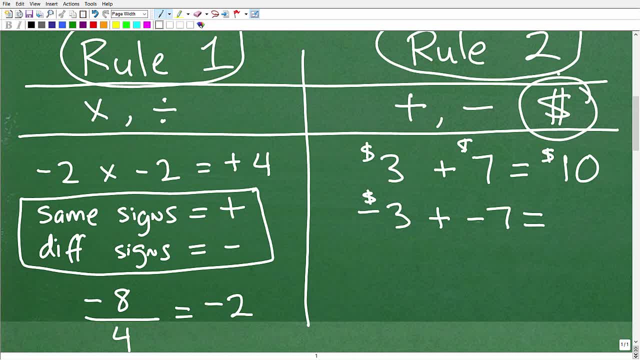 What does that mean? okay, to you all right? Well, it means that you have three dollars of debt. You don't really have money. You have less. You have no money. You have debt. right? Let's say, yeah, I have no money in my pockets and I actually owe somebody three dollars, right? 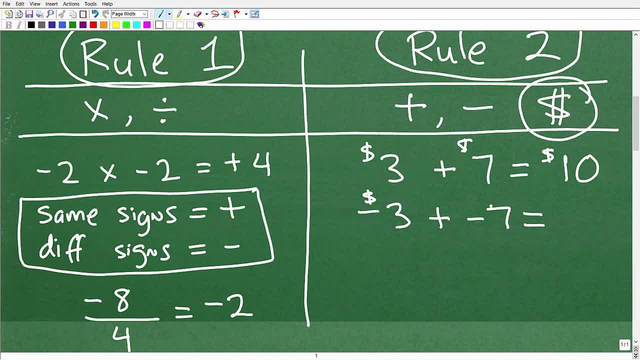 So that's what Negative three dollars means. And then you add another seven dollars in debt. So how much total debt do you have, right? So here you're, like One of your friends are like: hey, give me back my three dollars that I lent you. 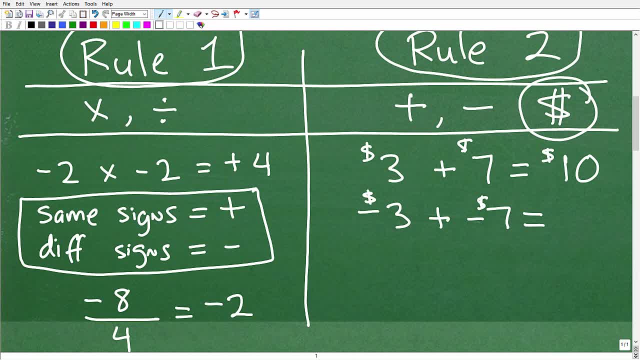 And you don't have any money, And then some other friend comes up to you and be like, oh yeah, give me my seven dollars that I lent you. You're like, oh man, in total debt I have this three and this seven. 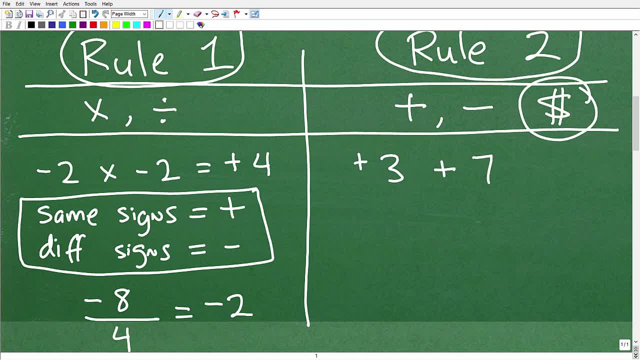 Okay, And we're going to add it to uh, seven. All right, So when we have a positive number, we don't need to write a little positive sign like this: So this is positive three plus a positive seven. So this is just simple addition, right. 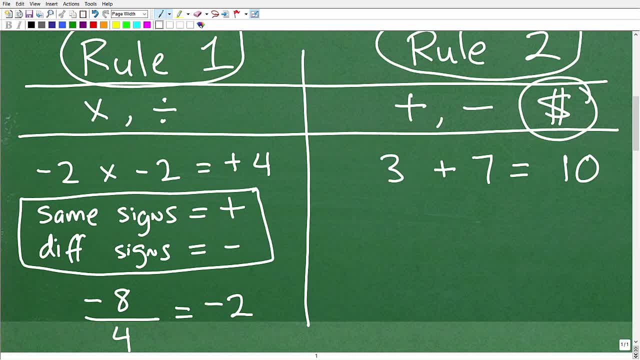 So the answer is 10.. Now I want you to think of this in terms of, uh, dollar situation. Okay, So this is like having $3.. Okay, At the end someone gives you $7.. So in total, you have $10. 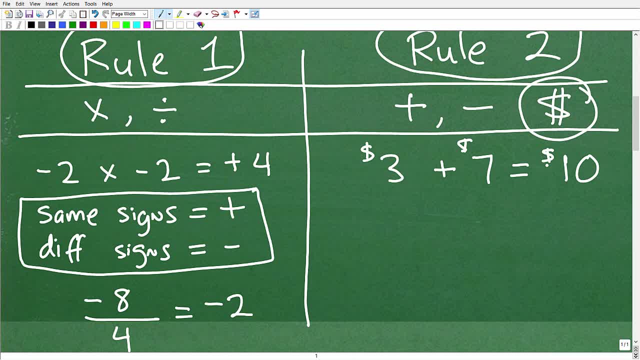 So that's pretty cool, Right? All right, Now let's kind of change this around. All right, Let's put: instead of uh having positive signs here, let's think of this, uh, in terms of negative signs. 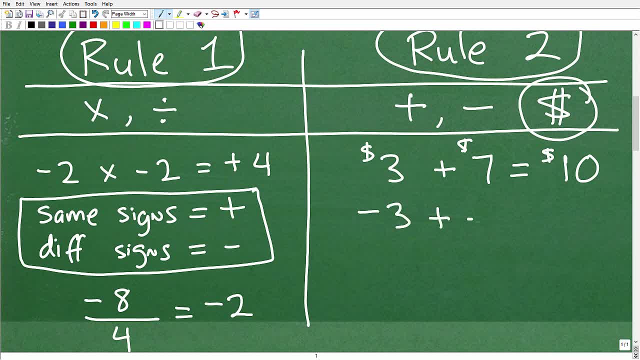 So let's have negative three Plus negative seven, And now let's figure out what this answer is going to be. Okay Now, negative three. right, If I have negative $3,. okay, Again, we're trying to use money here as our model. 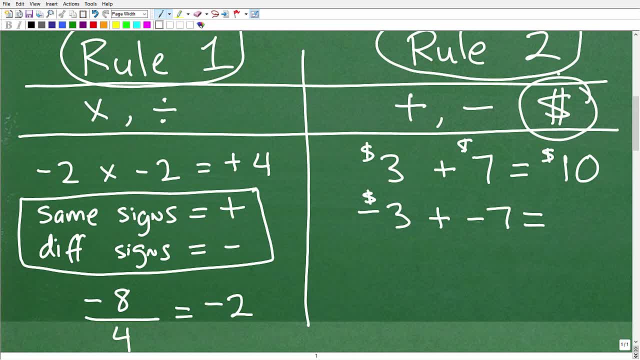 What is that mean? Okay To you, right? Well, it means that you have $3 of debt. You don't really have money. You have less. you have no money. You have debt. right, Let's say, yeah, I have no money in my pockets and I actually owe somebody $3.. 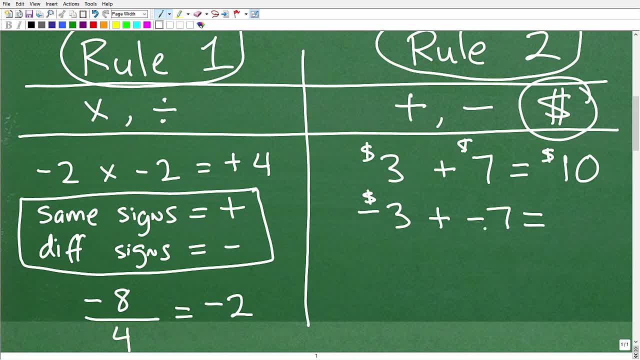 Right, So that's what negative $3.. $3 means. and then you add another $7 in debt. So how much total debt do you have, Right? So here you're, like one of your friends are like: Hey, give me back my $3 that I uh lent, you need to have. you don't have any money. 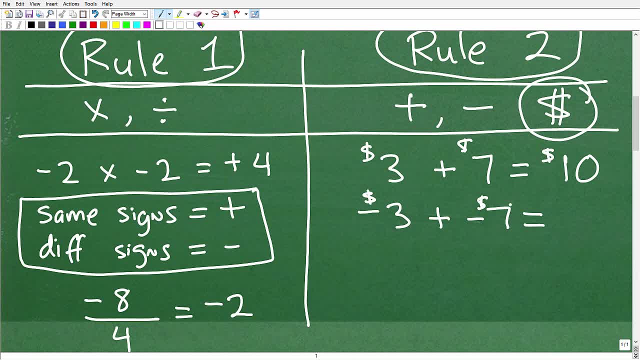 And then some other friend comes up to you and be like: oh yeah, give me my $7 that I lent you. You're like: oh, man, in total debt I have this three and the seven, So I have negative $10 in debt. 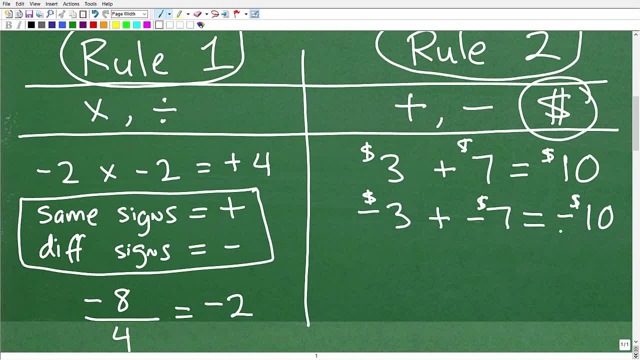 So negative three plus negative seven is negative 10.. Okay, So if you kind of remember that, you know when you're adding this or attracting uh positive and negative numbers. just think of uh it in terms of money. this is going to go a long, long way to uh help you avoid confusion. 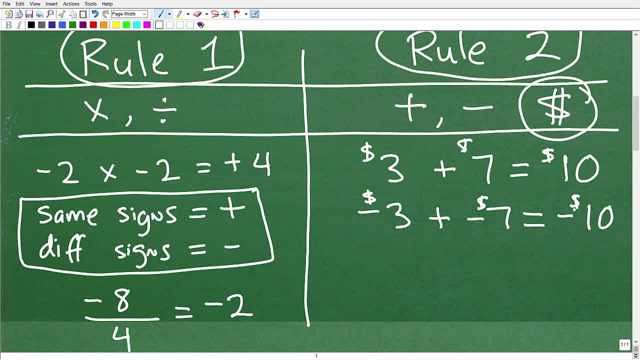 So I have negative ten dollars in debt. So negative three plus negative seven is negative ten. Okay, So if you kind of remember that you know when you're adding and subtracting positive and negative numbers, just think of it in terms of money. 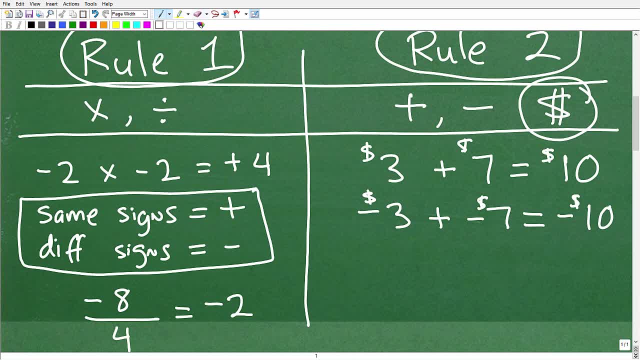 This is going to go a long, long way to help you avoid confusion. Now let's continue on with some more examples here. Okay, All right, What about? Let's say I have negative seven plus Three? Okay, So what do you think this is going to be? 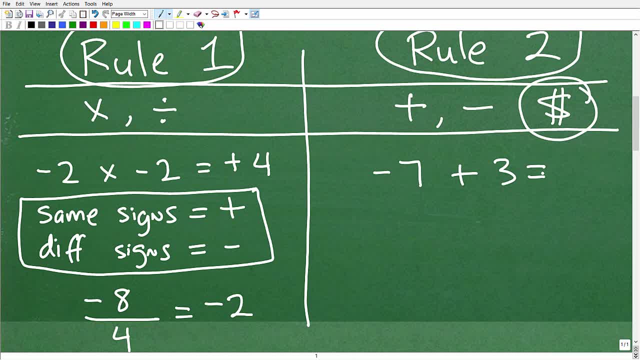 So if you feel like you got the concept down, all right, then you know, maybe go ahead and try to get this. you know, try to answer this, But negative seven plus three, this is like saying I have negative seven in debt. 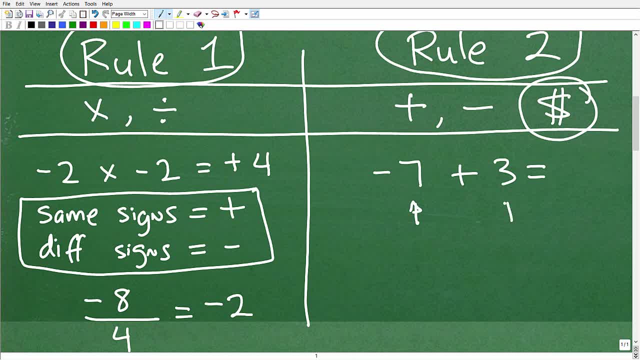 I owe somebody seven dollars, But then somebody gives me three dollars, right. So somebody gives me three bucks, like I have three dollars in my pocket, but I owe this person over here this seven dollars. So how much money do I actually have? 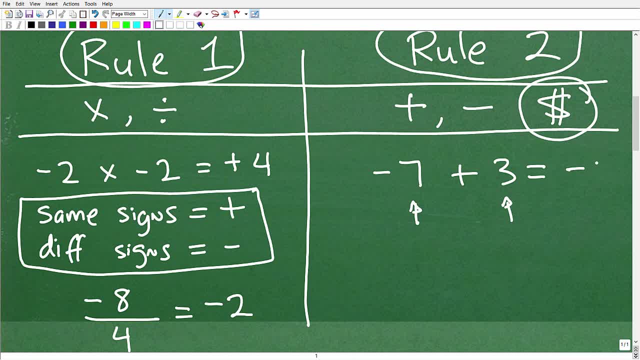 Well, I don't have any money, Okay, But my debt situation has improved. right, I give this three dollars to this person. Okay, All right, Hey, listen, I don't have all your money, but here's three bucks. 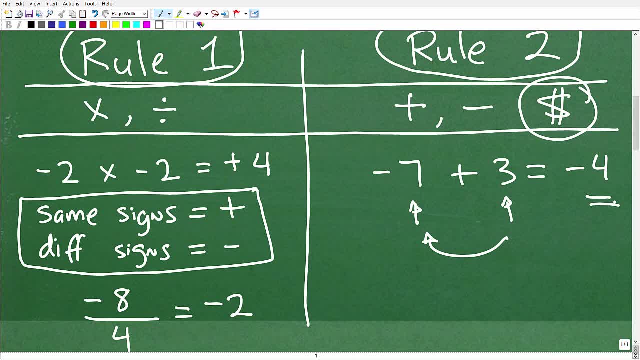 So what happens? Well, I still owe you four dollars, right? So negative seven plus three equals negative four, Okay, So hopefully you can kind of see the pattern here. Now. this number is larger, Okay, Meaning that this negative seven is larger than the positive three. 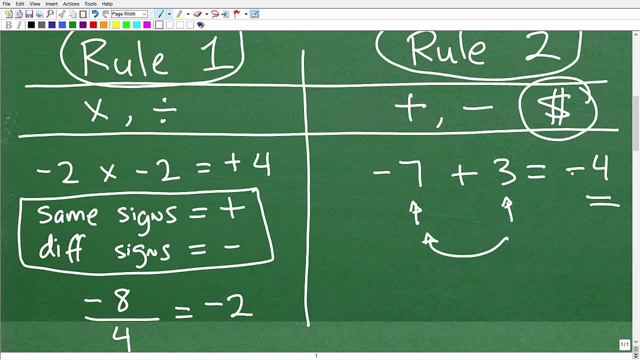 So our sign is negative. So when you're learning these rules, there's ways to think of a debt and you know to think of these rules in that manner. Okay, But all that really kind of means, if we use money as a model here, is that we have more debt than we have money. 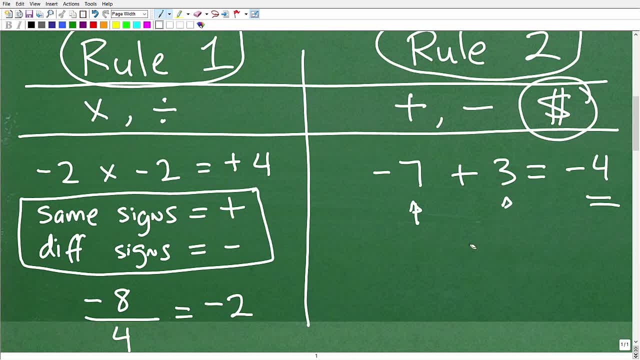 So we still have debt going on. Okay, All right, Now let's switch this around and let's do this problem. Seven plus Negative three: Okay. So what's the situation there? Well, here I have seven dollars. So, yay, I got seven dollars in my pocket. 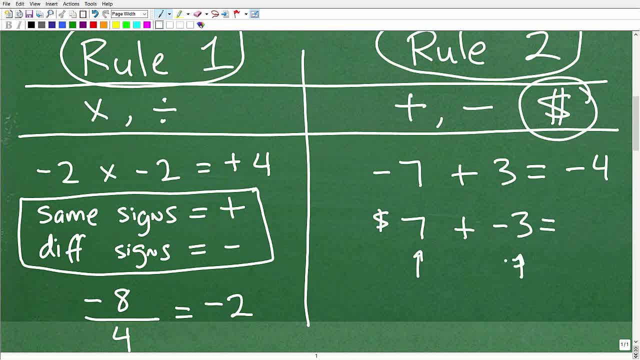 And one of my friends comes up and says: hey, where's my three bucks I lent you? You're like: oh, okay, I got you, I got you here, Let me give you those three dollars. Okay, After you give them those three dollars. 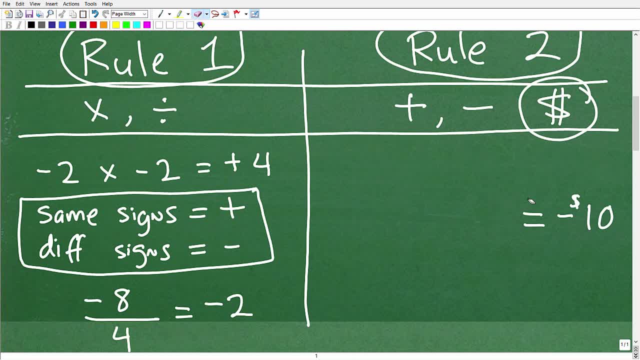 Now let's continue on with uh. some more examples here. Okay, All right, What about? uh, let's say I have negative seven plus three, So what do you think this is going to be? So if you feel like you got the concept down, all right, then, uh, you know, maybe go ahead and uh, try to get this. you know, try to answer this, but negative seven plus three. 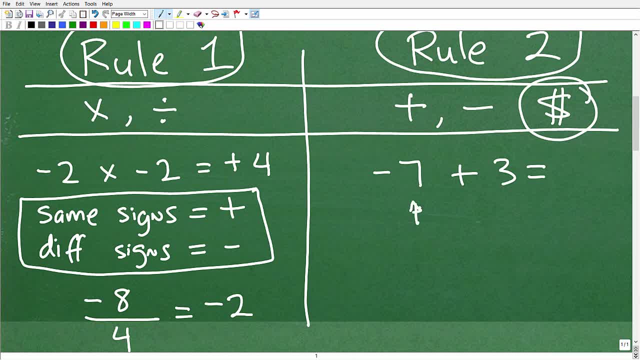 This is like saying: I have negative seven in debt, I owe somebody $7, but then somebody gives me $3, right? So somebody gives me three bucks, Like I have $3 in my pocket, but I owe this person over here, uh, this, uh, $7.. 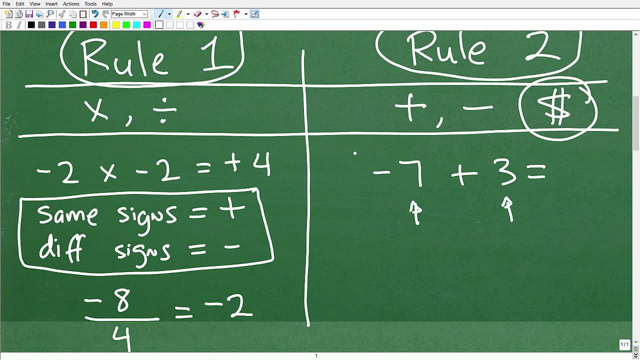 So how much Money Money do I actually have? Well, I don't have any money, Okay, But my debt situation has improved right, I give this $3 to this person, Okay, All right? Hey, listen, I don't have all your money, but here's three bucks. 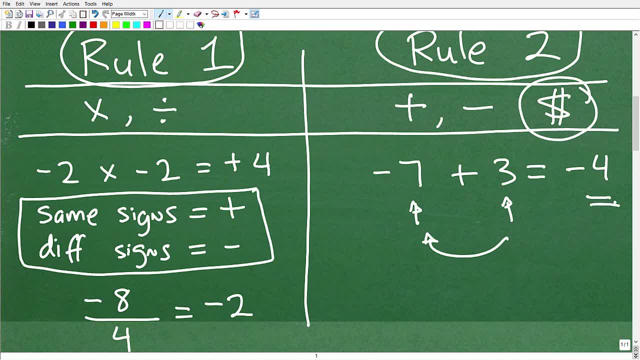 So what happens? Well, I still owe you $4, right? So negative seven plus three equals negative four, Okay, So hopefully you can kind of see the pattern here. Now it's this number is larger, Okay, Meaning that this negative seven is larger than the positive three. 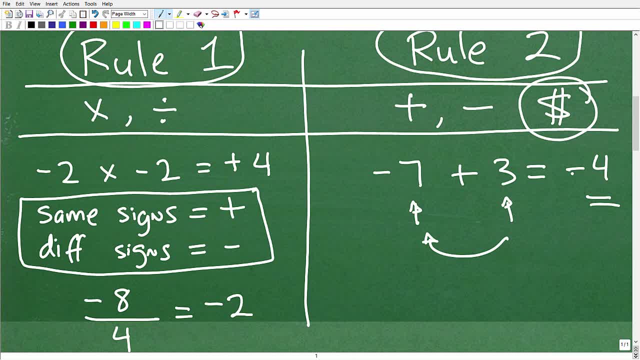 So our sign is negative. So when you're learning these rules, there's ways to think of a debt in it. you know to think of these rules in that manner. Okay, But that all that really kind of means if we're, if we use money as a model. here is 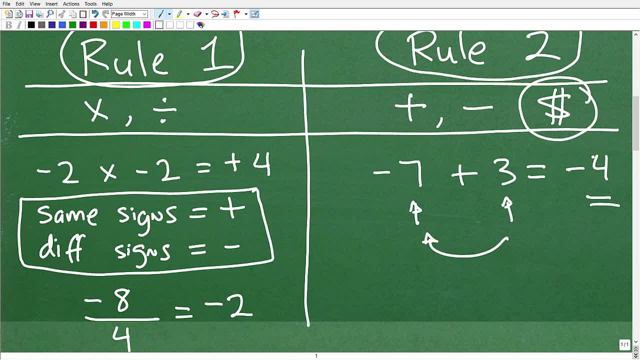 that we have more debt than we have money, So we still have debt going on. Okay, All right, Now let's switch this around and let's do this problem. Seven plus negative Three- Okay, So what's the situation there? 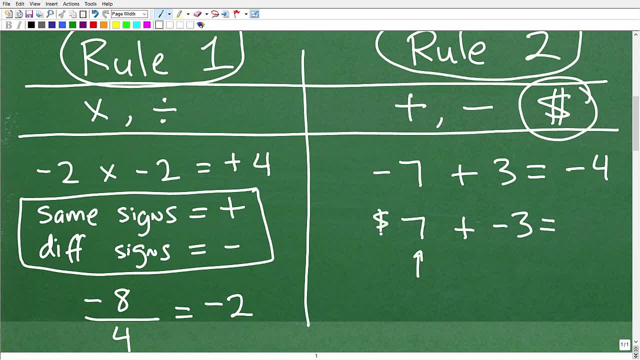 Well, here I have $7.. So, yay, I got $7 in my pocket. And one of my friends comes up and says: Hey, where's my three bucks I lent you. you know like: oh, okay, I got you. 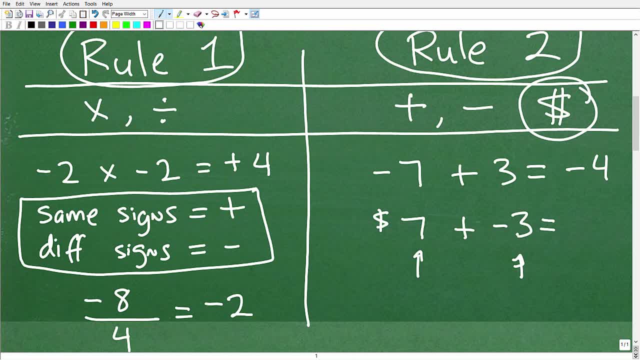 I got you here Can let me give you those $3. Okay, After you give them those $3. Okay, What do you have left? You have, uh, $4 remaining. Okay, Positive four, All right, And of course we would just write this as four. 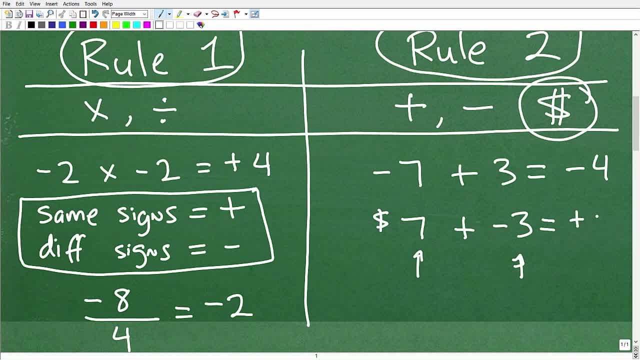 Okay, What do you have left? You have four dollars remaining. Okay, Positive four, All right, And of course we would just write this: And As four, All right. So Hopefully you're kind of getting the idea here. 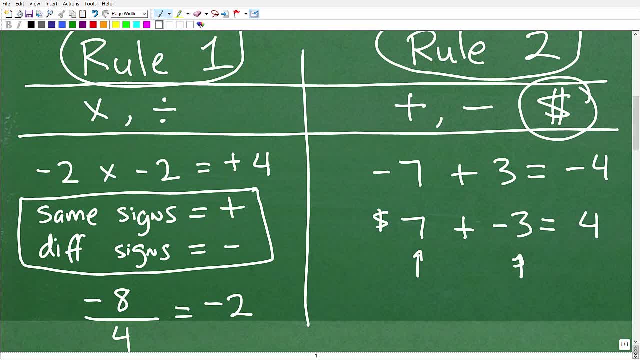 Right, So okay, And this is not too bad. So if you always think of this in terms of money, you'll be okay. Now let's kind of put another twist on this And really talk about the subtraction situation. So let's say, I have three minus seven. 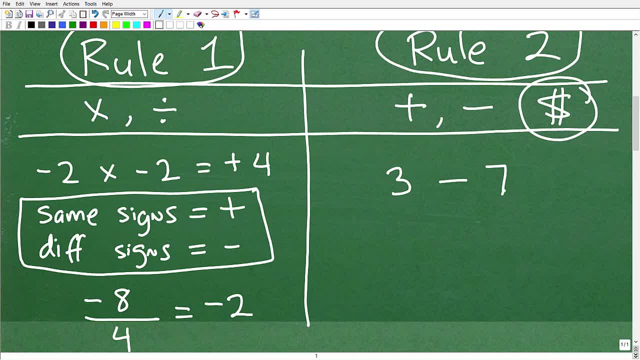 All right, Three minus seven, Okay, Now here You know, what we've been doing before is just addition. You know we are of examples involved addition operators. So what we want to do is take this problem, Okay, And think of it in another way. 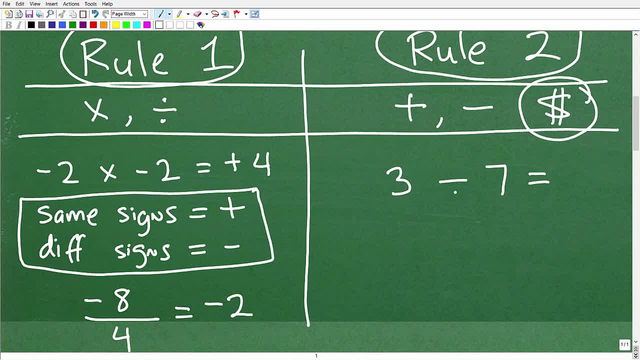 All right, And this is what we call plus negative. So what I want you to do is this subtraction sign: Okay, I want you to turn it into an addition sign. Okay, All right, So you're going to take the subtraction sign. 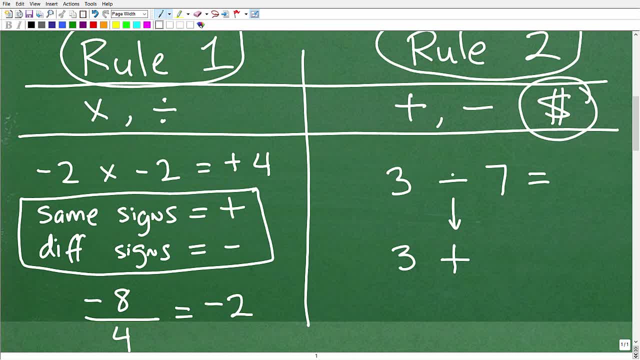 Turn it into addition. You're like, hey, what's going on, though? What we're going to do is take this subtraction sign and we're going to put it right here, Boop. Okay. So we're going to take the subtraction sign, this operator, turn it into addition sign. 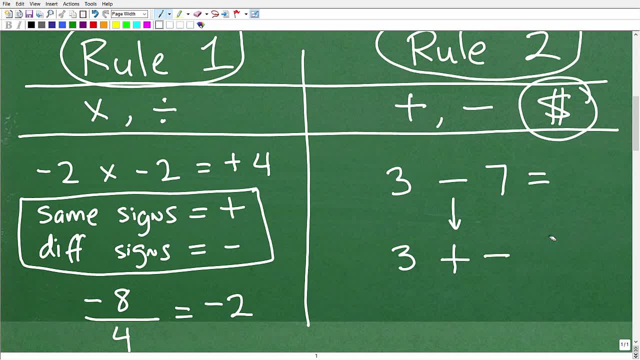 but then put this right here in front of the seven: Okay, Let's write that a little bit better Like so. So, actually kind of do it. Let's make it a little bit more like this: Negative seven. So three minus seven is equivalent to the problem three plus. 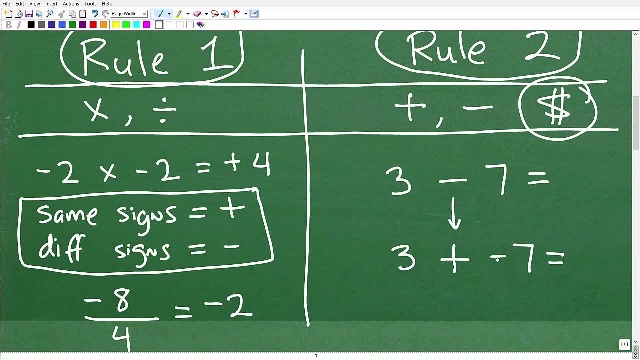 Negative seven. Okay, So here, what's the situation? Well, you have $3,, but you owe somebody $7. Okay, So what's your financial situation? Well, you still owe $4.. Okay More: You still have $4 of debt. 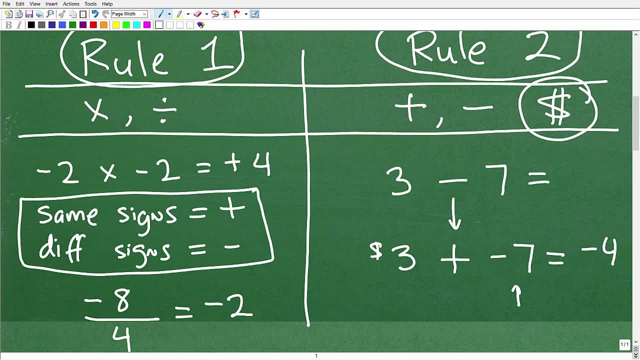 Okay. So I can go on and on with more examples, but if you understand these two rules, this is kind of do a quick Recap. Okay, So we're dealing with a multiplication and division. It's the same rule, Okay. 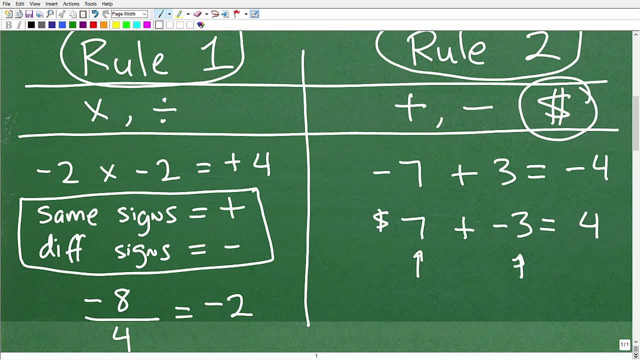 All right. So hopefully you're kind of getting the idea here right. So okay, And this is not too bad. So if you always think of this in terms of money, you'll be okay. Now let's kind of put another twist on this and really talk about, uh, uh, the subtraction situation. 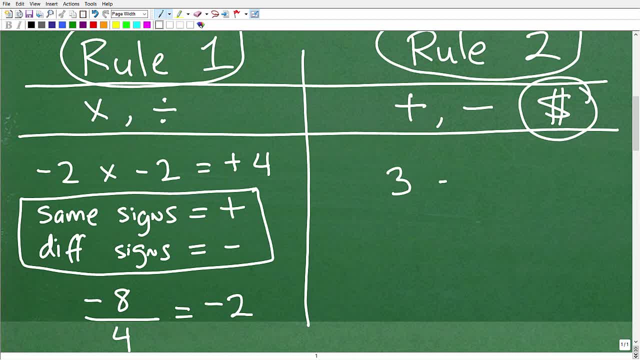 So let's say I have, uh, three minus seven. All right, Three minus seven, Okay, Now here you know what we've been doing. Okay, What we've been doing before is just addition. you know, we, we, uh are of examples involved. 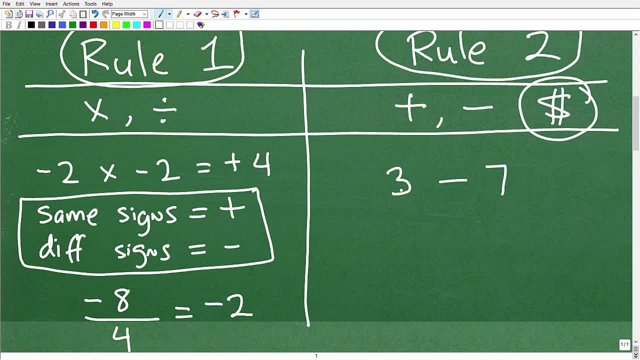 addition operators. So what we want to do is take this problem, Okay, And think of it in another way. All right, And this is what we call plus negative. So what I want you to do is this subtraction sign: Okay, I want you to turn it into an addition sign. 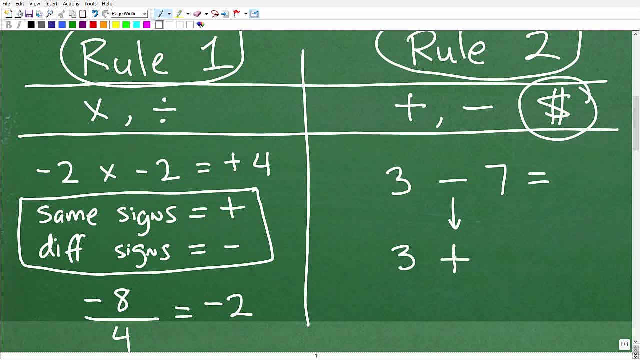 Okay, All right. So you're going to take the subtraction sign, turn it into addition sign. You're like, Hey, what's going on? So what we're going to do is take this, uh, this, this subtraction sign, and we're going. 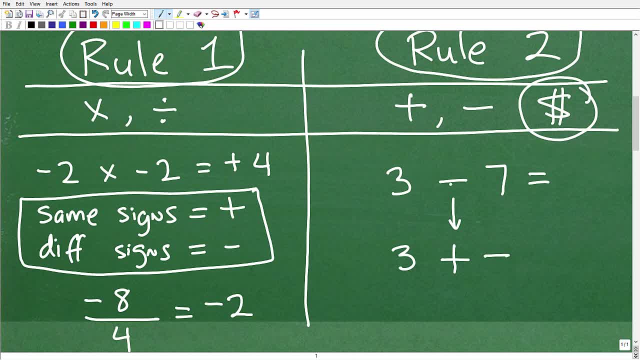 to put it right here: Boop. Okay, So we're going to take the subtraction sign, this operator, turn it into addition sign, but then put this right here in front of the seven: Okay, And let's write that a little bit better. 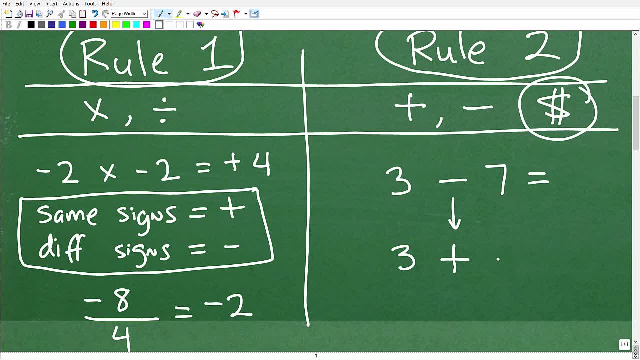 Like so. so it actually kind of do. let's make it a little bit more like this: negative seven. So three minus seven is equivalent to the problem Three plus negative seven. Okay, So here what's the situation? Well, you have $3, but you owe somebody $7.. 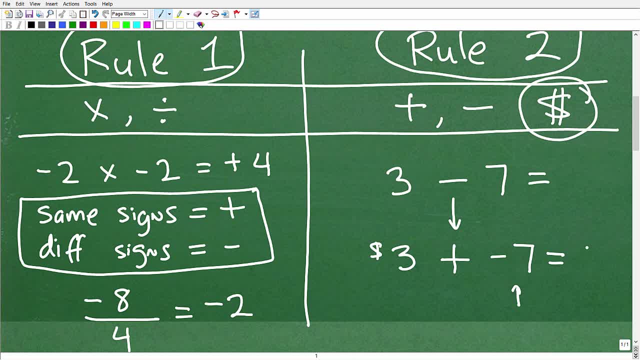 Okay, So what's your financial situation? Well, you still owe $4.. Okay More: you're still have $4 of debt. Okay, So I can go on and on with more examples, but if you understand these two rules, this 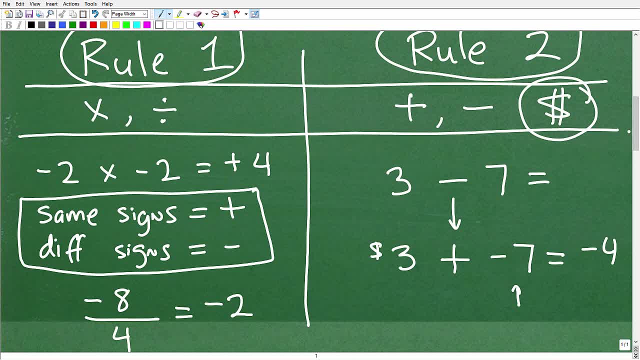 is kind of: uh, do a quick recap. Okay, So we're dealing with a multiplication and division. It's the same rule, Okay, So same signs, All right. Negative and negative or positive, positive answers. Positive goes for both division and multiplication. 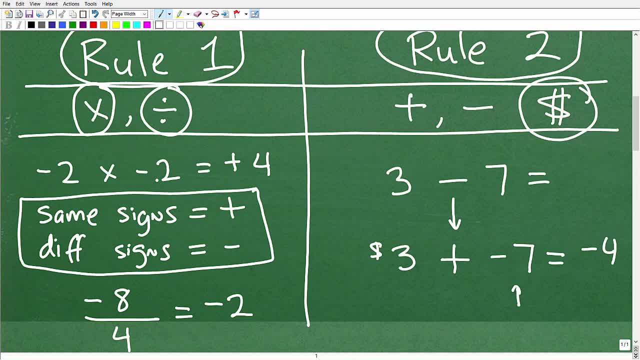 So same signs, All right. Negative and negative, or positive, positive answers. Positive goes for both division and multiplication. If you have different signs going on, the final answer will be negative. Very simple, Okay. Rule number two: we'll call it the money rule, right? 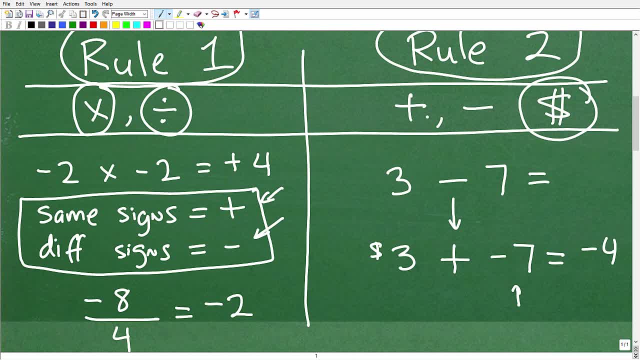 So it applies for both adding and subtracting, positive and negative numbers, And we talked about You know how to think of numbers in terms of money, if you will. And the one big thing with subtraction is we're going to take subtraction problems and turn them into addition problems by doing this little plus negative. 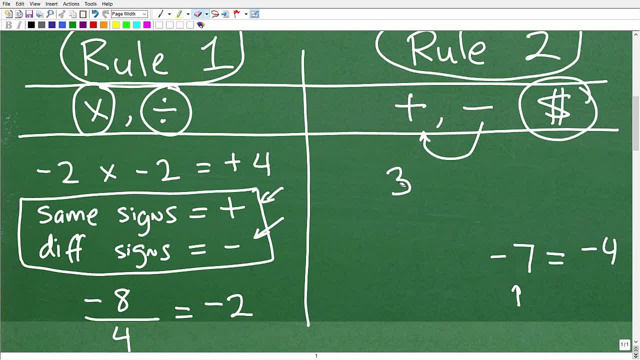 Now one little thing here. Let's just kind of do one last thing. Okay, I don't want to leave you without all the mathematical you know rules that you really want to know. So let's say we had two minus. 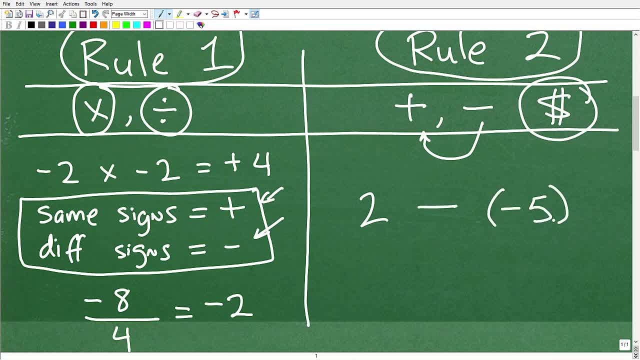 Let's say, Let's say, a negative five. Okay, So how do we handle that situation? Well, we'll still want to do this little plus negative. So it would be like two plus a minus of a minus five, Okay, So just to make sure, 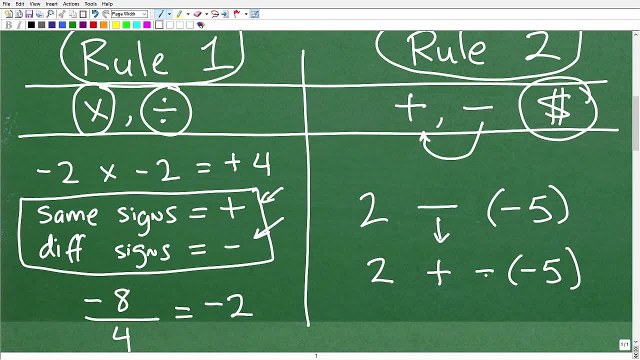 Okay, there's no confusion out there. A negative of a negative five, Oftentimes a negative sign in mathematics is we can think of it as being the opposite. So what's the opposite of a negative five? That is going to be a positive five. 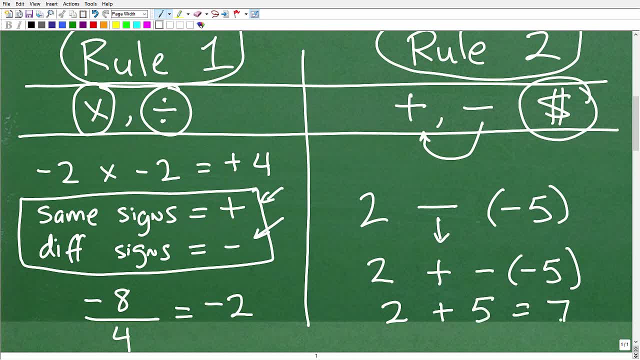 So that would be two, That's going to be two plus five, And of course we know that's going to be seven. Okay, So of course this second rule has more variations going on, but it's not difficult, Okay. 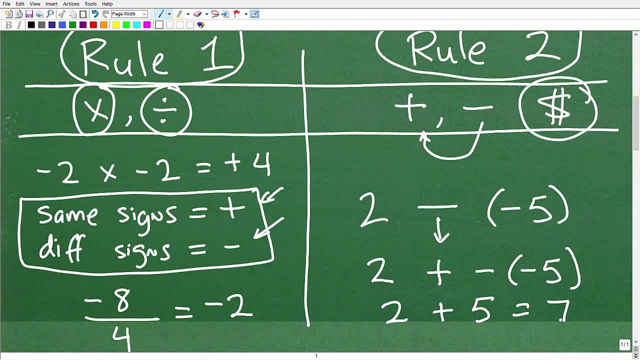 You got to. you know, don't, If you're learning in math, Okay, The key is this: Don't try to learn math by just memory. Okay, It's not going to work. You know? just being like: oh, I got to memorize all these different crazy rules. 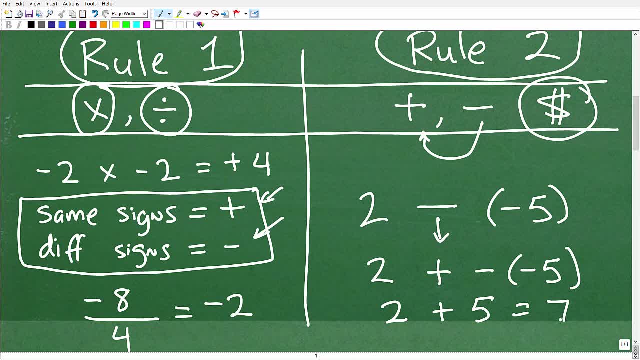 And if you don't understand the rules and you're trying to memorize them, you're definitely going to make a mistake. So that's why I try to memorize all these different crazy rules. I try to you know, explain these concepts in easy ways for you to understand. 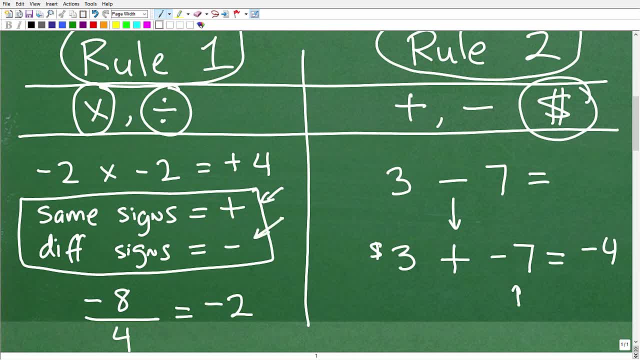 If you have different signs going on, the final answer will be negative. Very simple, Okay. Rule number two: we'll call it the money rule, right? So it applies for both adding and subtracting positive and negative numbers. And we talked about- uh, you know. 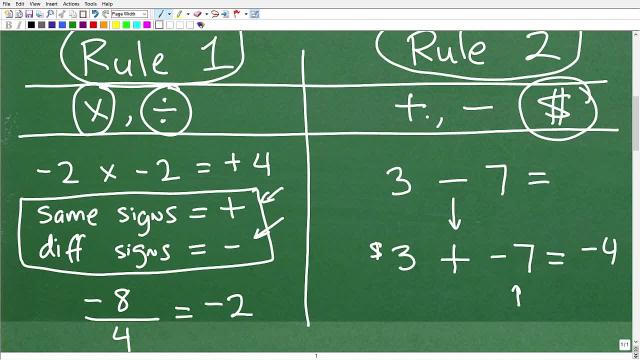 how to think of numbers in terms of money, if you will. And the one big thing with subtraction is: we're going to take subtraction problems and turn them into addition problems by doing this little plus negative. Now, one little thing here. let's just kind of do one last thing. 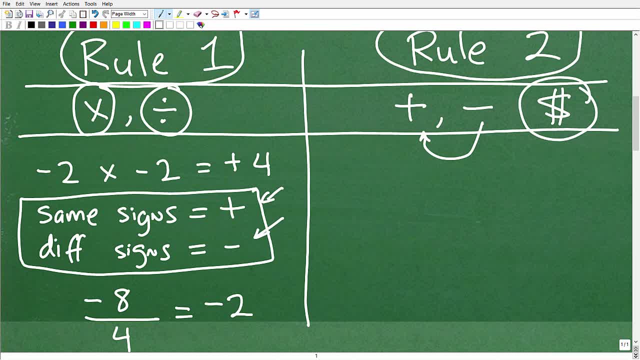 Okay, I don't want to leave you without all the mathematical- uh, you know rules that you really want to know. So let's say, let's say we had two minus, let's say a negative Five, Okay, So how do we handle that situation? 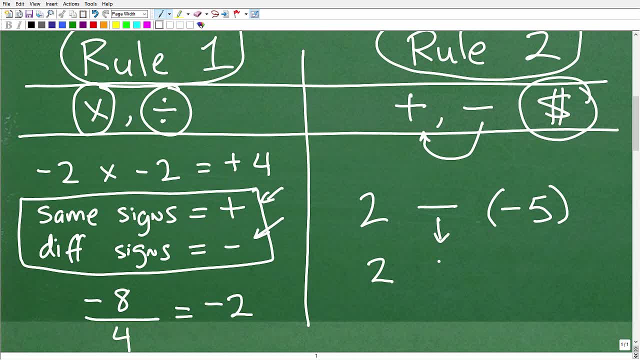 Well, we'll still want to do this little plus negative. So it would be like two plus a minus of a minus five. Okay, So just to make sure, okay, there's no confusion out there. A negative of a negative five. 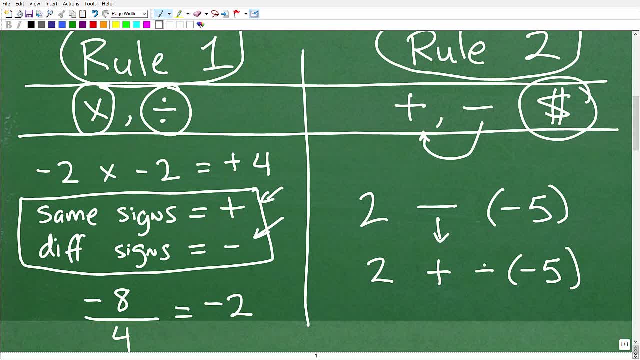 Oftentimes a negative sign at mathematics is: we can think of it as being the opposite. So what's the opposite of a negative five? that is going to be a positive five, So that'd be two plus five, And of course we know that's going to be seven. 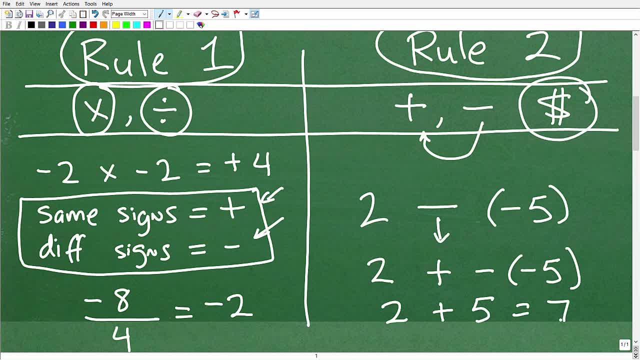 Okay. So of course, his second rule has more variations going on, but it's not difficult. Okay, You got to. you know, don't? if you're learning in math, okay, The key is this: don't try to learn math by just memory. 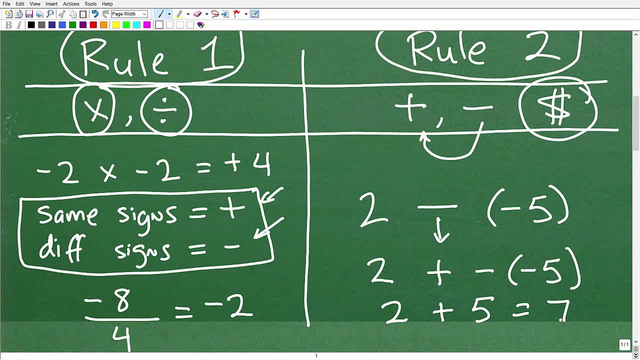 Okay, It's not going to work. you know just being like: oh, I got to memorize all these different crazy rules. And if you don't understand the rules and you're trying to memorize them, you're definitely going to make a mistake. 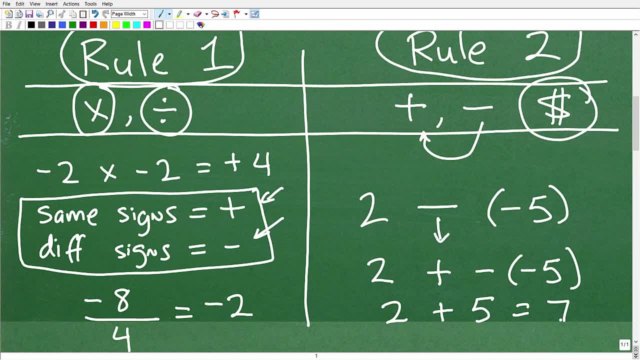 So that's why I try to uh, you know- explain these Okay Concepts and easy ways for you to understand. So hopefully this uh video helps you out, If you can get these rules down and never again make a mistake with your positive